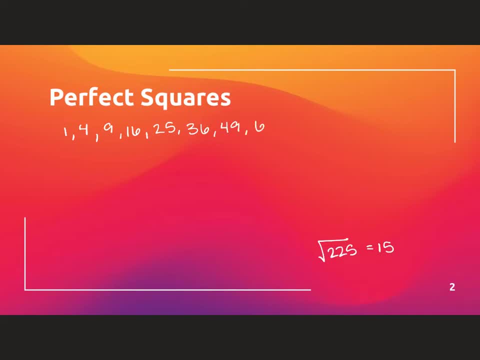 8 times 8 is 64.. 9 times 9 is 81.. 10 times 10 is 100.. 11 times 11 is 121.. 12 times 12 is 144.. 13 times 13 is 169.. 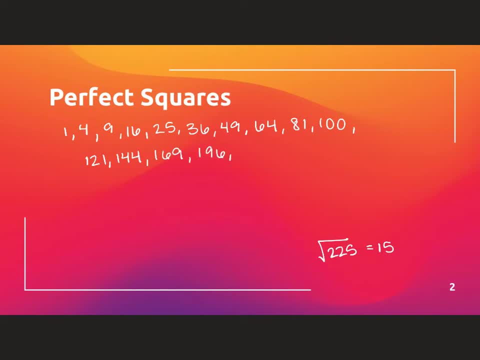 14 times 14 is 196. And 15 times 15 is 225.. We won't really go much beyond that, but I like to go all the way up to 225.. A lot of people ask me: okay, well, how can you remember all those? 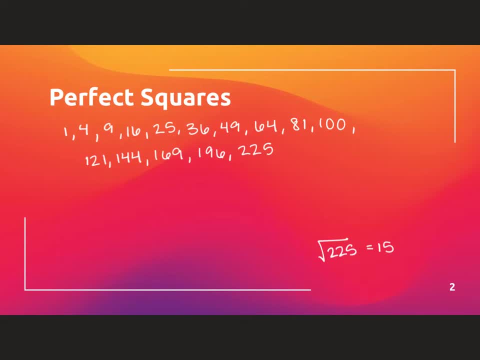 Remember, all I did was I just went through and I multiplied, you know, 1 times 1,, 2 times 2,, 3 times 3,, 4 times 4, etc. all the way down the line. So that's how I do it, That's how I memorize those. 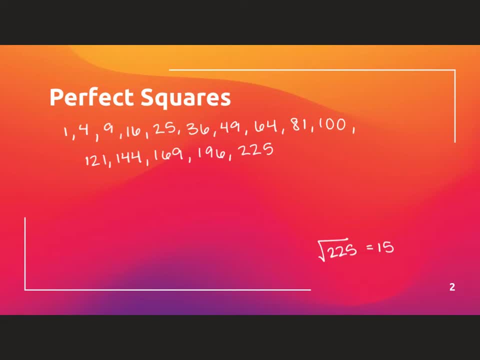 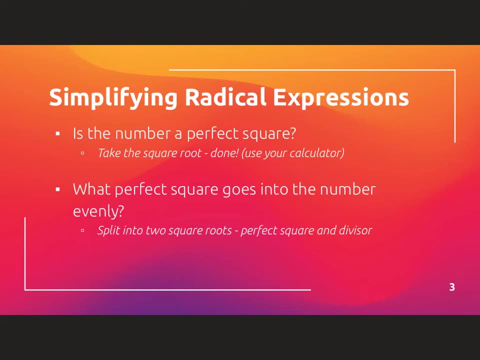 So, when we're talking about simplifying radical expressions, we need to know those squares. There's perfect squares in order to simplify these. So our questions that we're going to ask ourselves is the number a perfect square? So if, for instance, you are given a problem that looks like this: 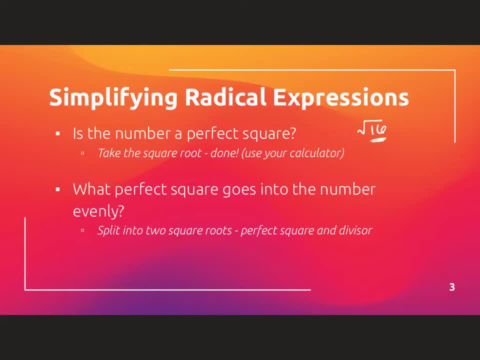 and I ask you to simplify that- this number, this number beneath it, is a perfect square. So then you just take the square root of it and then you're done. Use your calculator if you need to. It's okay to not know all the perfect squares. 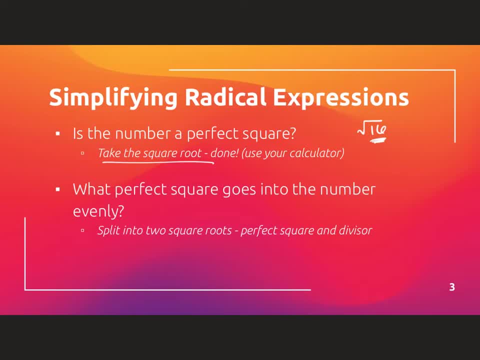 or at least what the square roots are. but you should know, you should be able to identify them. Okay, If it's not a perfect square, then you have to do a little bit more work. And then you have to ask yourself: 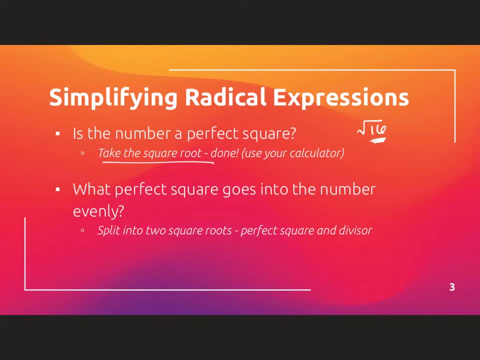 what perfect square goes into the number evenly? And what you'll do then is you're going to split it into two square roots. One will be a perfect square and one will be, well, not a perfect square. Okay, And then, last but not least, our very last question is: 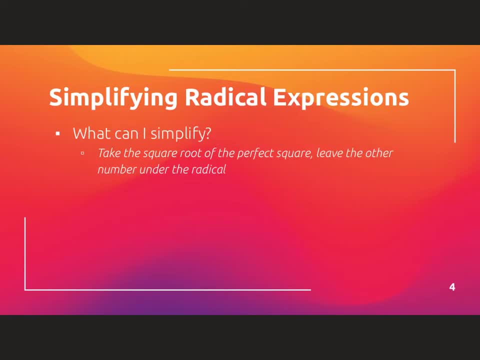 what can I simplify? Basically, all you're going to do is take the square root of the perfect square and you're going to leave the other number unnoticed. You're going to leave it underneath the radical or the square root. If you don't know that a radical means square root. 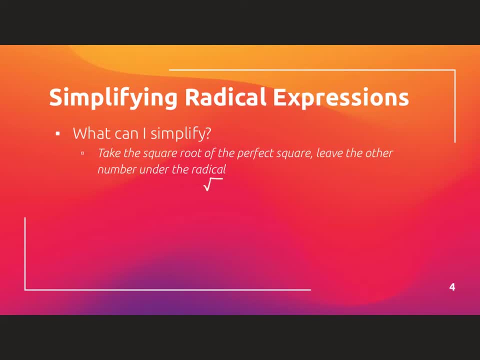 maybe draw yourself a little picture or write yourself a little note, just so you remember that. Let's go ahead and look at a few examples here. Okay, so I have the square root of 121.. 121 is on my perfect square list. 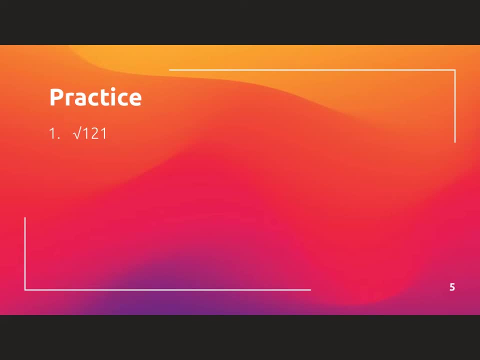 This is a perfect square. So if you type in square root of 121 on your calculator- and if you need me to help, you find that I'm happy to do so- you should get 11. And then we're done. That's how we simplify those types of questions. 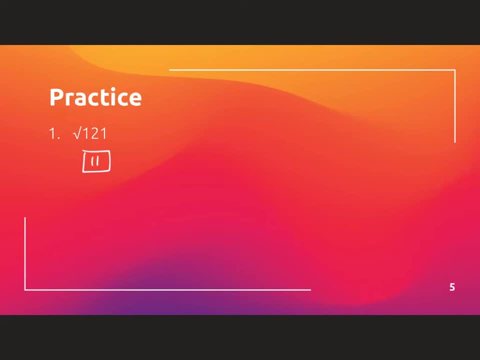 Okay, So 11 is my final answer for number one. Let's look at number two, A square root of 50.. 50 is not on my perfect square list. 49 is, which is really close to 50, but it's not quite. 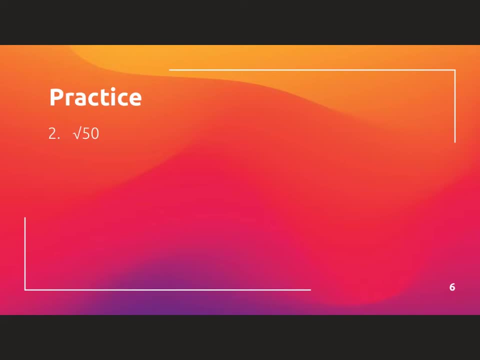 So, when we are looking at simplifying these, what we like to do is we need to find the largest perfect square that will go into this. So, if you remember, my list had numbers like 1,, 4,, 9,, 16,, 25,, 36,, 49,, 64, right. 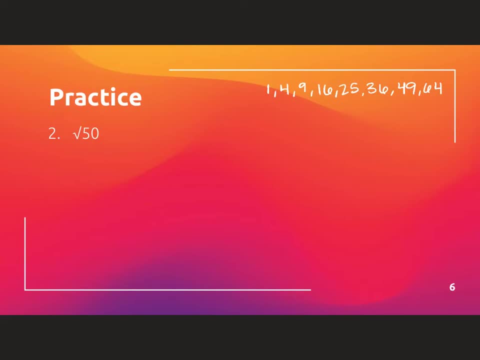 So those are all the numbers that are on my list. Now. 50 is right here. right, It's right in between 49 and 64, which means I can't use anything that's bigger than 49.. So now I'm just going to start typing into my calculator. 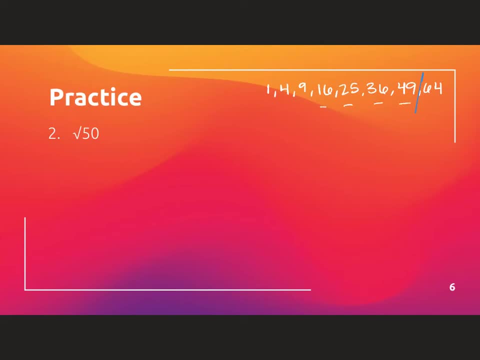 50. 50 divided by all of those numbers- okay. So if I do 50 divided by 49, I get a decimal. I don't want a decimal, okay. So 49 does not work. I try 50 divided by 36.. 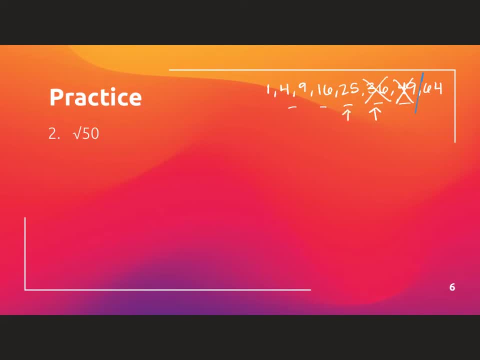 That gives me a decimal. It doesn't work. Then I try 50 divided by 25, and I get 2.. That is a whole number. That is what I'm looking for. So my two numbers that I'm looking for are going to be 25 and 2.. 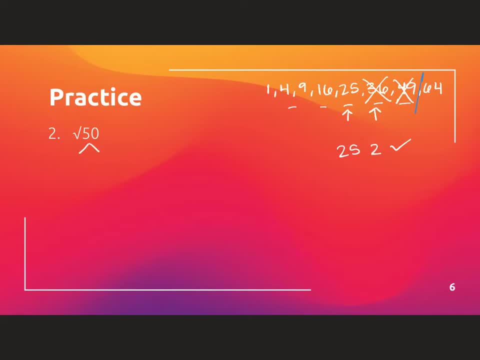 What I'm going to do is I'm going to split this up, okay. So over here on the left, I'm going to put my perfect square: That's 25.. That was the number that was on my list, okay. 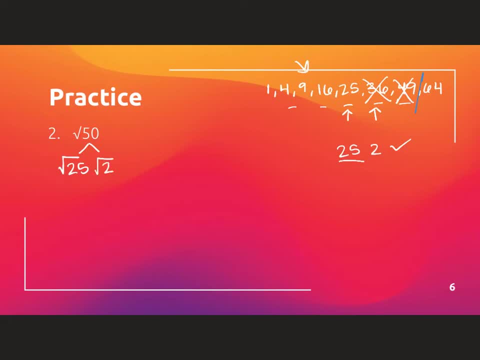 On the right side I'm going to put 2.. That was the other number I had. That's the number I had to times 25 by to get back to 50. So if you take 25 and you times it by 2,. 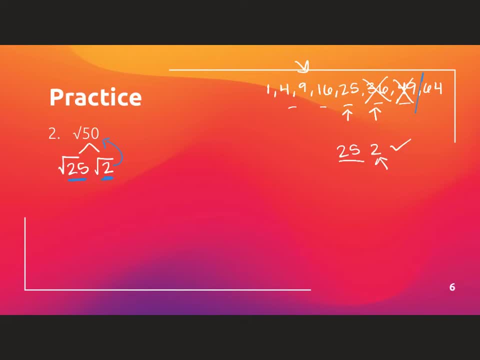 you should end up with that number. If you multiply these two- two numbers that are underneath the square root- you should always end up back with your original number. Okay, So now what I'm going to do is I'm going to take this first number. 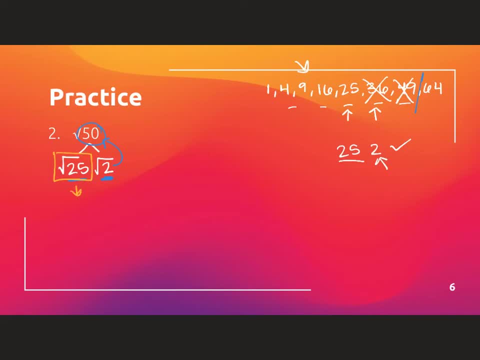 which should be a perfect square, and I'm going to take the square root of it. That's going to give me 5.. If you try taking the square root of 2, you are going to get a decimal. We don't want to deal with that. 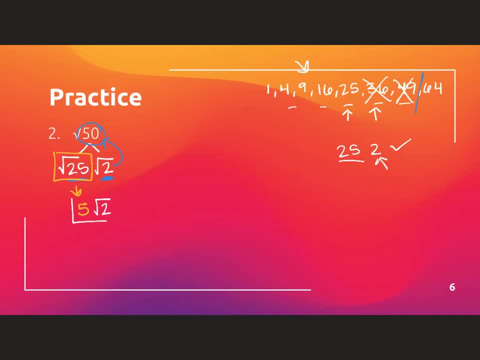 So we're going to leave this as the square root of 2.. This is my final answer. It looks a little weird, but this is what we mean by simplifying. We want an exact answer, nothing rounded like what you would have if you took the square root of 2.. 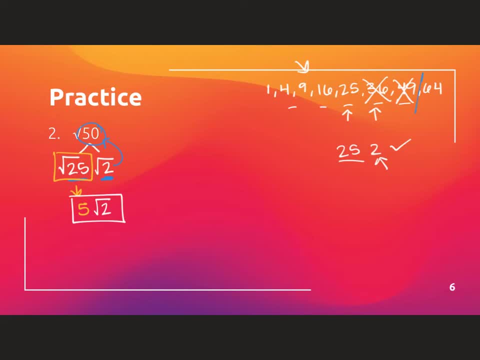 If you have any questions about this, please let me know and I'd be happy to walk you through it. Let's go ahead and look at number 3, square root of 48.. So again, 48 is not on my list. 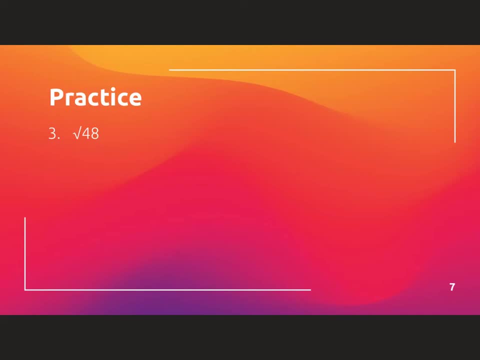 so I have to run through. So my square roots, or my perfect squares, were 1, 4, 9,, 16,, 25,, 36,, 49.. I can't go any bigger than that, because 48 is right there in the middle. 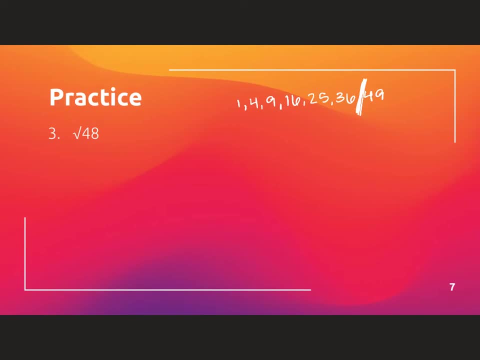 So I'm just going to keep trying some numbers. So I'll try. you know, 48 divided by 36.. That one doesn't work. Let's do 48 divided by 25.. That one does not work. 48 divided by 16.. 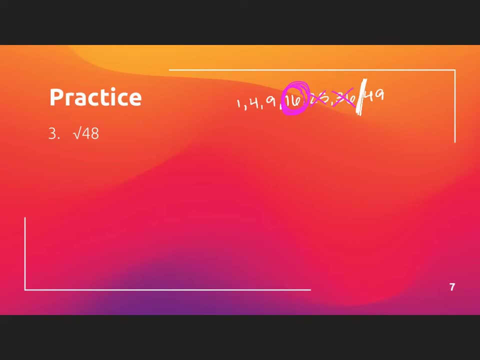 This one does work. It's going to be 16 and 3.. So that's what I'm going to use when I split this up. I'm going to put the square root of 16 first, because that's the number that was on my list of. 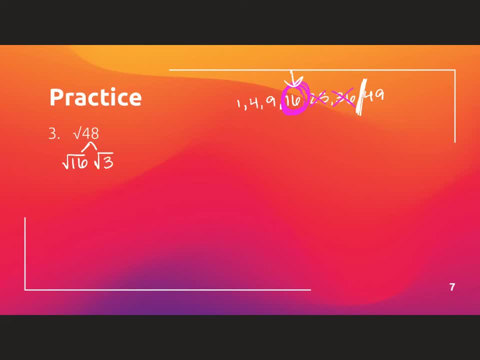 perfect squares, and then the number that I had to multiply by to get 48, that one goes next. So remember: this number times. the second number here should always bring me back to that original number: 16 times 3 gives me 48.. 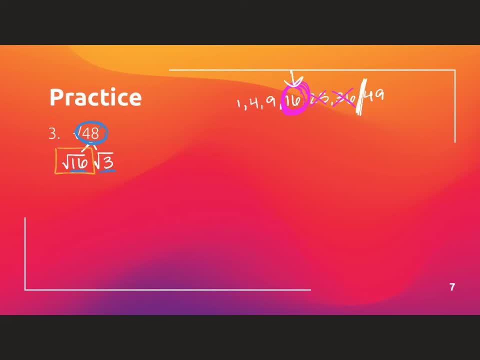 And now again, that first number should be your perfect square. The square root of 16 is 4, and then I can't do anything with that 3,, so I'm just going to drop that down, And that's my final answer. 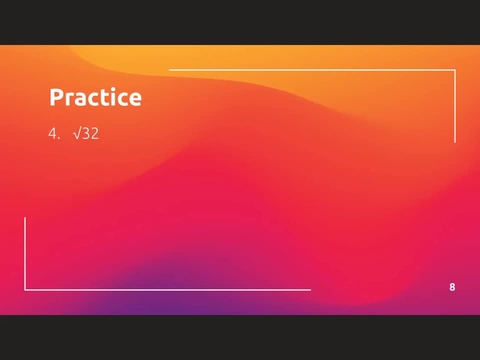 Again, please let me know if you have any questions. All right, number 4.. So, again, not on my perfect square list. So I've got 1,, 4,, 9,, 16,, 25,, 36,. 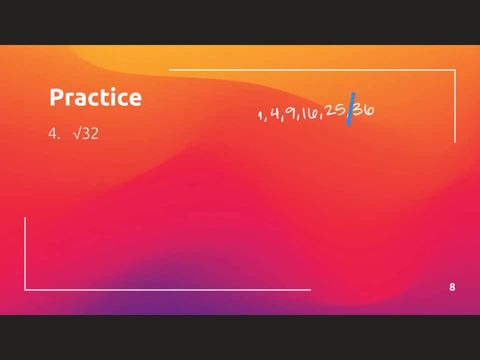 and I don't need to go any farther because my number's right there in the middle. You are going to get very good at recognizing. you know which numbers go into which- like which perfect squares go into which numbers. But for right now I'm going to go with 4.. 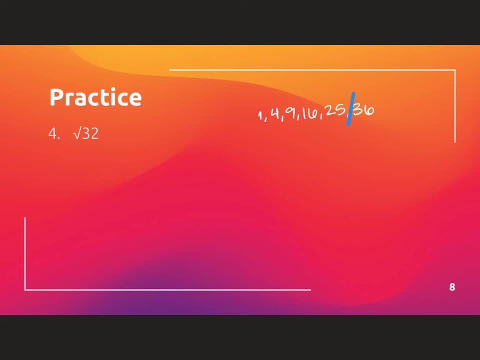 Now, you might be a little new to this, and that's okay. So if I start looking, I'm going to do 32 divided by 25.. That gives me a decimal which does not work. I'm going to do 32 divided by 16,. 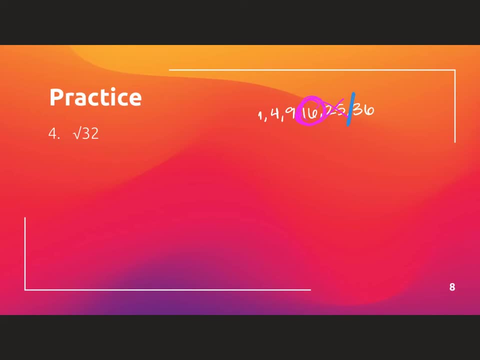 which gives me 2.. That is not a decimal, so 16 is the number I want again. So I'm going to split this up. Remember: 16 goes first because it's the perfect square and the number I had to multiply by to get back to 32 goes second. 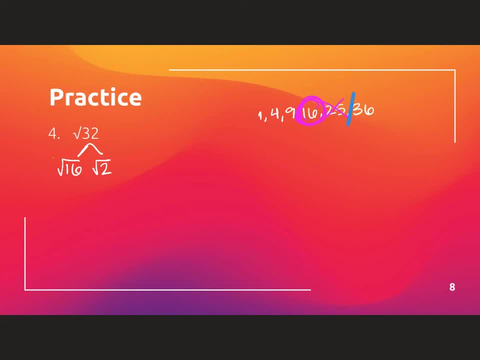 which was 2.. Okay, So my first number again should be a perfect square. If I take the square root of that, I get 4, and then I'm just going to drop that square root of 2 down, since I can't do anything with it. 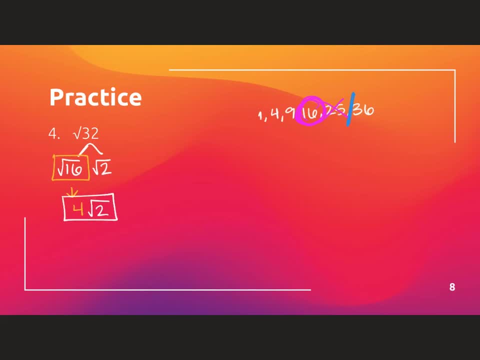 So 4 times the square root of 2, and that's my final answer, Number 5.. If I look at my list of perfect squares, 64 is actually on that list, So I can go ahead and take the square root of 64,. 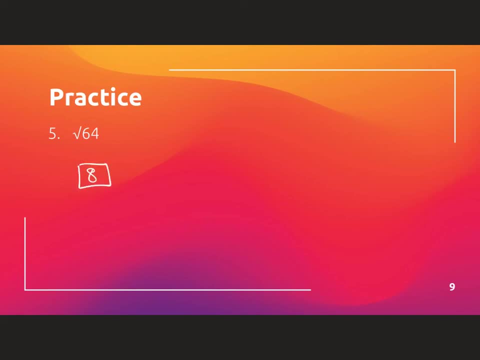 and I should end up with 8, and I am done. I don't need to do anything with simplifying it with other square roots, I just get my whole answer, Number 6.. I would like you to try on your own real quick. 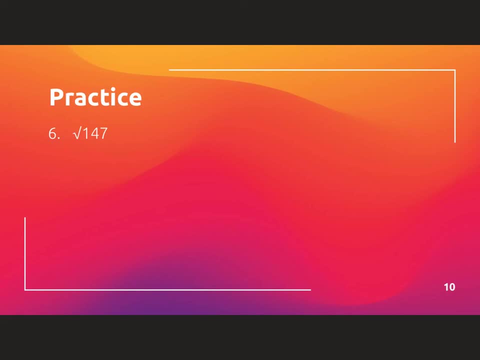 So go ahead and figure out where 147 is on your list of perfect squares and then simplify it down. Then you can come back and check your answer, Alright? so when I did this, I ended up with 7 root 3, or 7 times the square root of 3.. 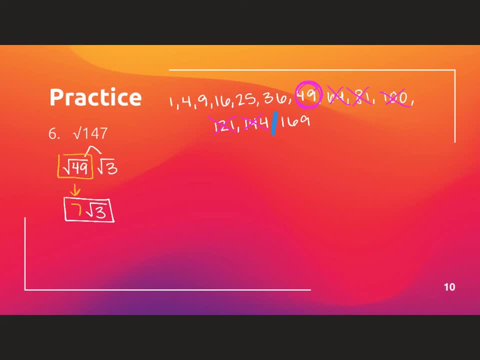 If you got something different or you're not sure how I got here, please just let me know and I'm happy to again walk through it with you. But again, this is why I tend to go so high on my list of perfect squares.